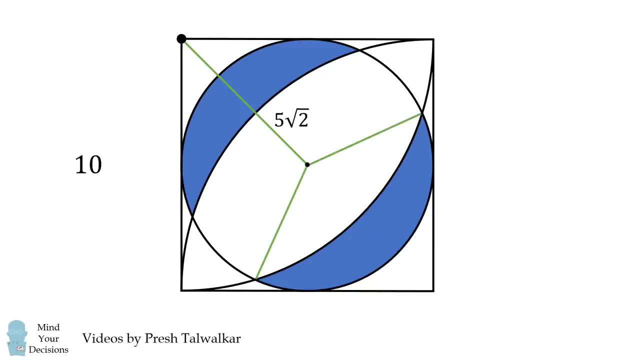 Next, we'll draw radii of the inscribed circle. Since the inscribed circle has a diameter of 10, its radius will be 5.. Now we'll draw radii of this quarter circle. It'll have a length of 10, because it's exactly the same length as the side of the square. 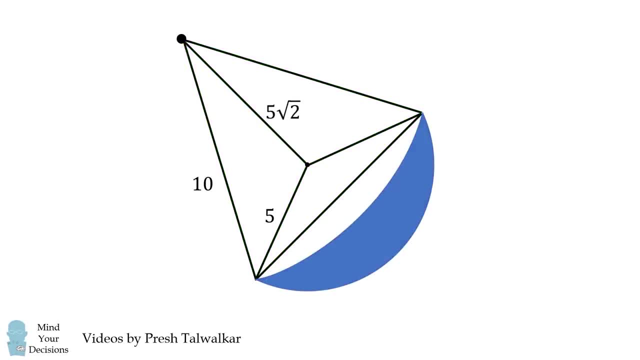 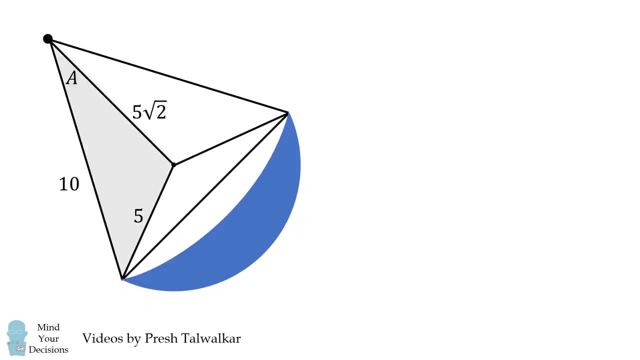 Finally, we'll draw this chord. Let's now focus on one of the triangles in this diagram. We know all three sides of the triangle, so let's solve for this angle A. We'll use Al-Kashi's law of cosines. We'll substitute in the values we have for this triangle and then solve for the angle A. 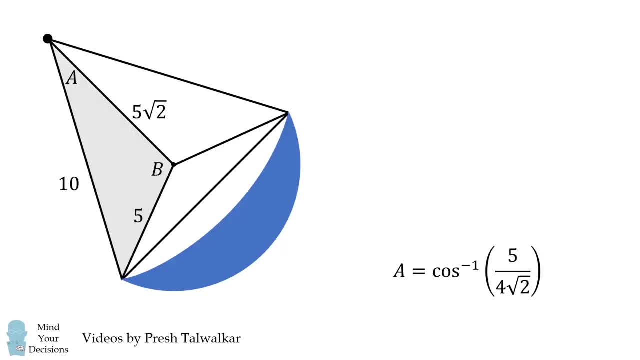 We'll put that to the side, and now we'll solve for this angle B. We'll again use Al-Kashi's law of cosines. We'll substitute in the values for this triangle and then we'll solve for the value of A. 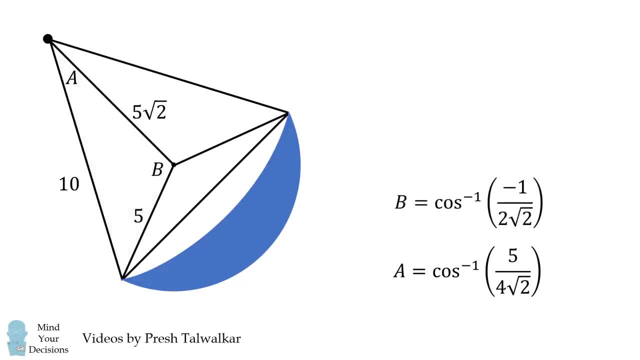 We'll use Al-Kashi's law of cosines. We'll substitute in the values for this triangle and then we'll solve for the angle B. Now notice that by symmetry this is also angle B, so this will be C, which is equal to 2 pi minus 2B. 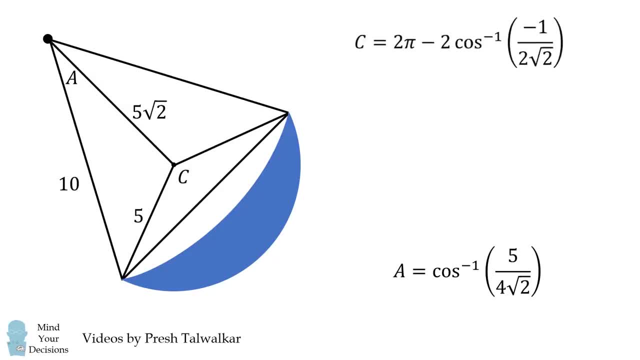 We'll calculate the angle C Again by symmetry. this is angle A, so we can solve for the value of 2A. We'll now calculate the area of this circular sector. We'll then subtract the area of this circular sector. 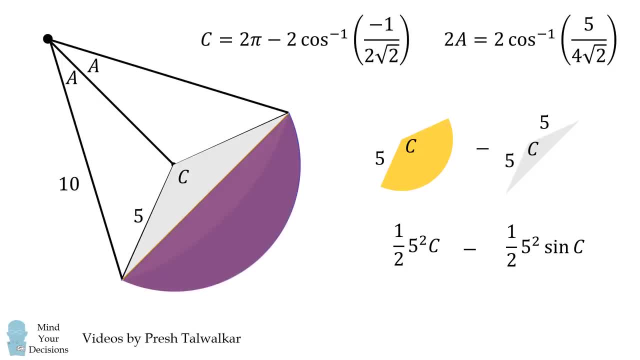 We'll get the area of this triangle and we'll get the area of this circular segment. We'll simplify this a little bit and we'll put it to the side. We'll now calculate the area of this circular sector and then subtract the area of this following triangle and 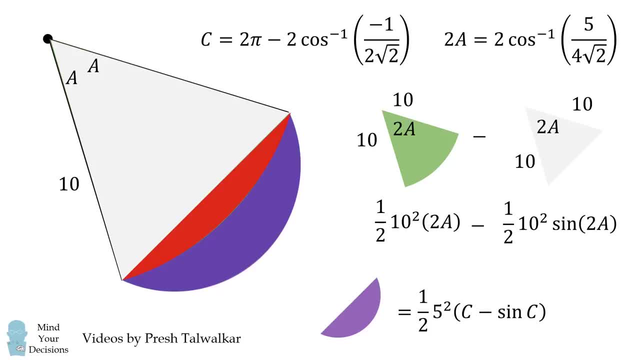 then we'll get the area of this circular segment in red. We get this formula and then we'll simplify it, And now we want to take the area of this red shape from the area of this purple shape. So that'll be pretty much our answer. 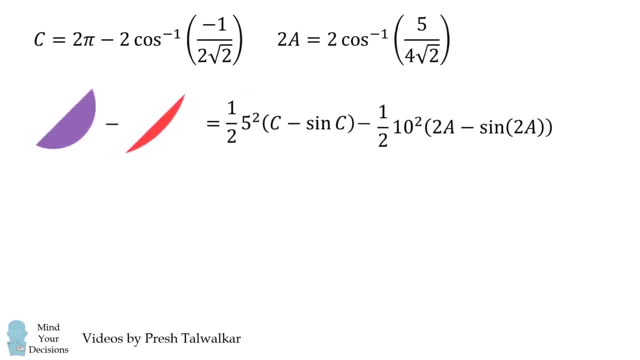 We'll subtract the red shape from the purple shape. But just for fun, let's simplify this a little bit. We have the sine of c, so we'll substitute in the value for c, We'll use some trigonometric identities and then we'll use the double angle identity. 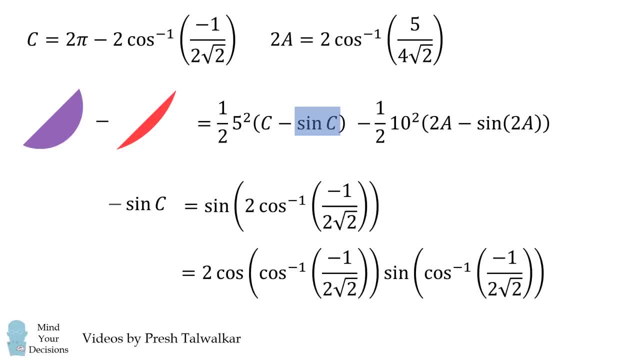 Sine of two times an angle will be two times the cosine of the angle multiplied by the sine of the angle, The cosine of the inverse cosine of a quantity. we'll simplify. Then we have the sine of the inverse cosine of a quantity. 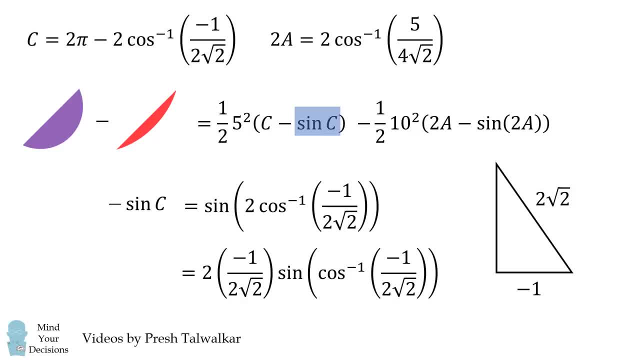 We can draw a right triangle. This is the value of the cosine in this triangle. so we can solve for the sine of the angle. and we substitute that in, So we simplify this and we figure out what sine of c is equal to. 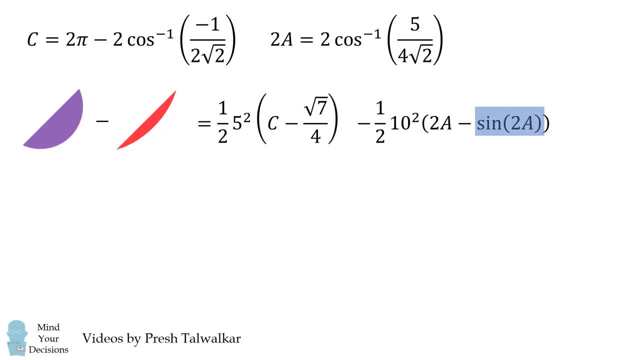 We'll substitute that and then we'll do the same sort of thing for sine of two times a. We'll use some trigonometric identities, Then we'll simplify and then we'll draw a triangle and we'll again calculate the sine of this triangle. 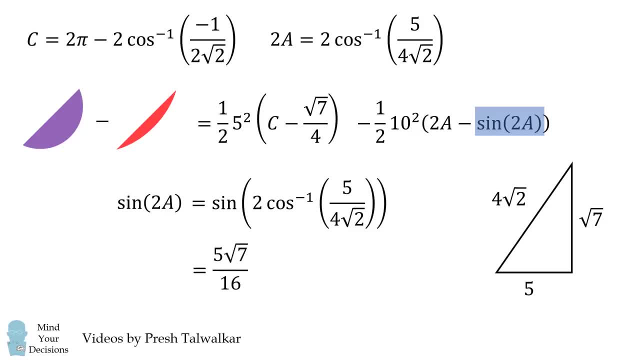 This allows us to simplify even further and we get what sine of 2a is equal to. Now, when we take the red shape from the purple shape, we end up with the blue shape, But we need the value of two of these blue shapes, so we'll multiply everything by two. 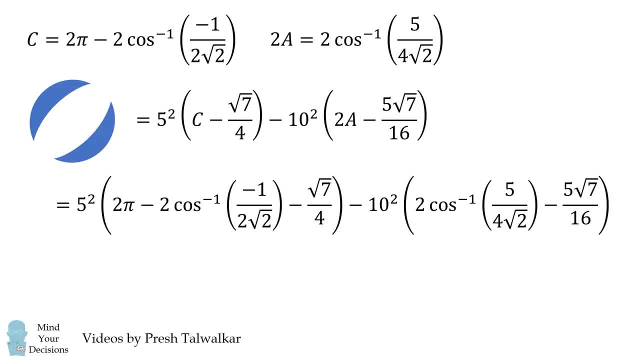 Next, we can substitute in our values of c and j, of c and a, and then we'll simplify and we end up with this exact form of the answer, and this is approximately 29.276, and don't forget the square centimeters. and that's our answer now at this. 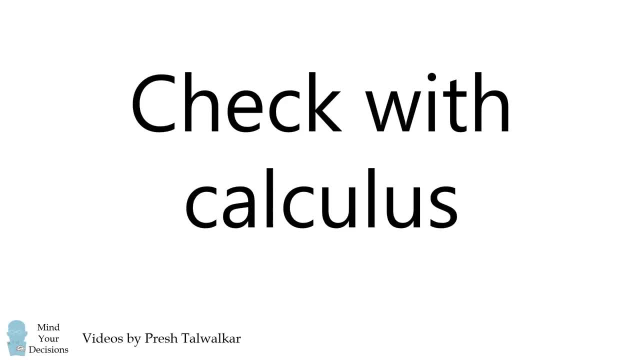 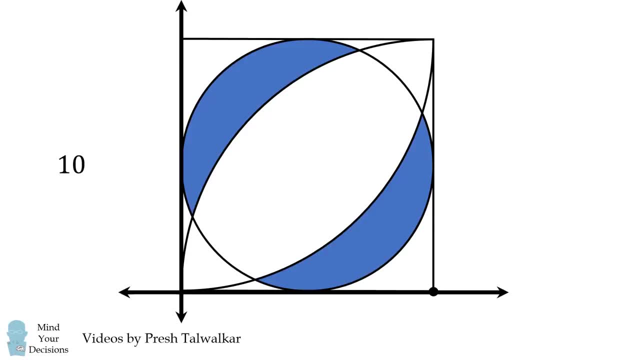 point. we've done a lot of work, so it'll always be good to check your answer, and we're going to check it using calculus. so we have our shape and we'll put a coordinate system in place. we'll then put this point as 10 comma 0. we'll then calculate the equation of this arc. then we have the equation of: 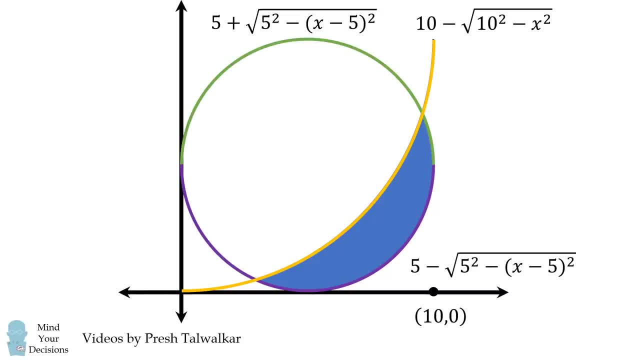 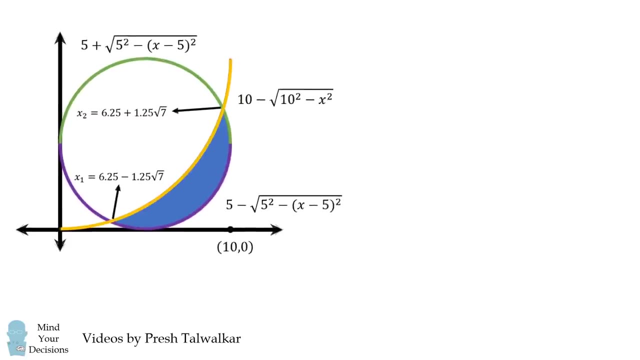 this lower part of the circle and then the equation of this upper part of the circle. we can then calculate the intersection of the lower part of the circle with this quarter circle and then we calculate the intersection of this upper circle with the quarter circle. we now have three functions and we can calculate the area as follows. 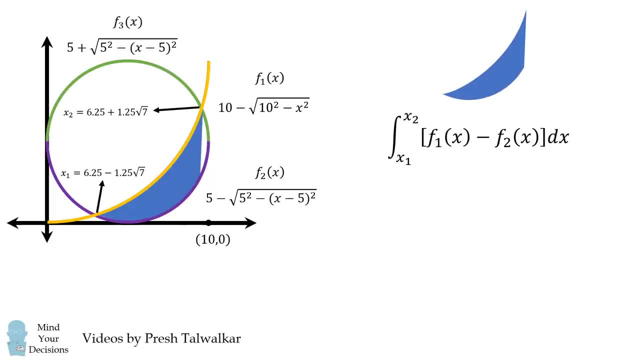 so the first part of the shape will be the integral that's going from x1 to x2 of f of 1 minus f of 2.. the remaining will be the integral that goes from x2 to 10 of f of 3 minus f of 2..